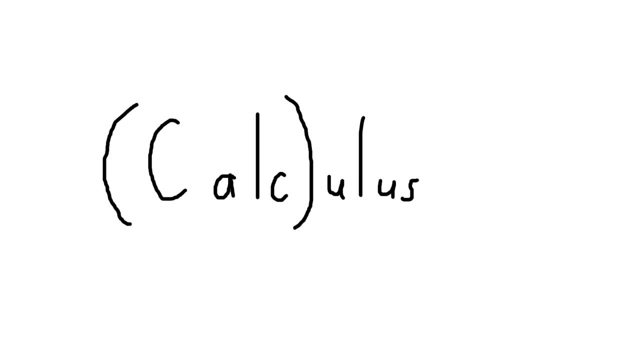 Calculus time. Calculus, or just calc, also known as the biggest barrier to cross over to the pure math zone, is the mathematical study of change. Specifically, it means change over the course of something. Most often, this something is time, but it can be anything like distance or time. Let x. 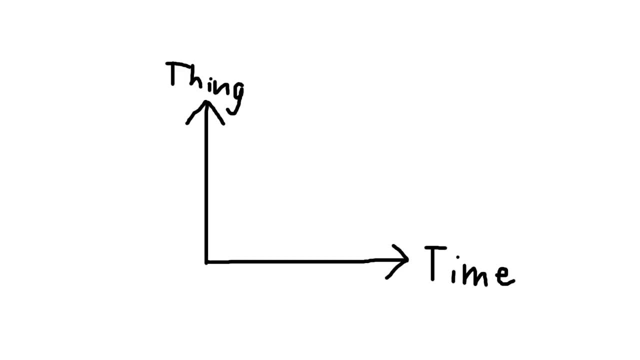 be time and y be the thing we want to measure. For a graph like y equals x. for every one we move to the right, we move one up, So the slope is one. But what if we had a wacky graph like this? Well, 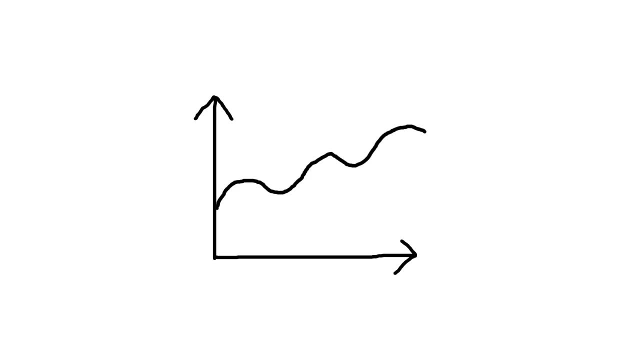 we can't answer that, but we can answer for the graphs like this. But first we need to learn about limits. Limits are pretty boring when the expression follows usual rules of math. Limits are a way of making exceptions to rules. For example, we can't divide by zero, but with limits 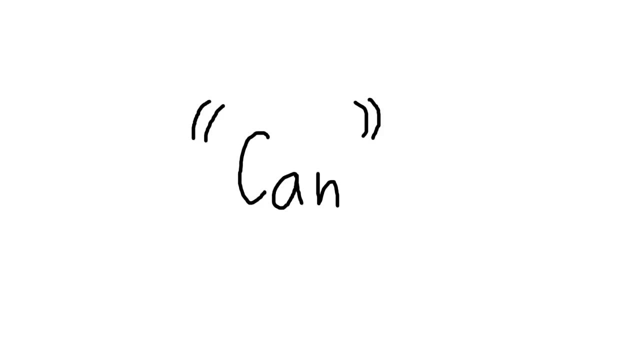 we can divide by zero. Let's write out this limit, as x approaches zero, of five divided by x. Technically, we're not dividing by zero, We're dividing by a number so small that it might as well be zero. This is what's called infinitesimally small. So what's five divided by a? ridiculously. 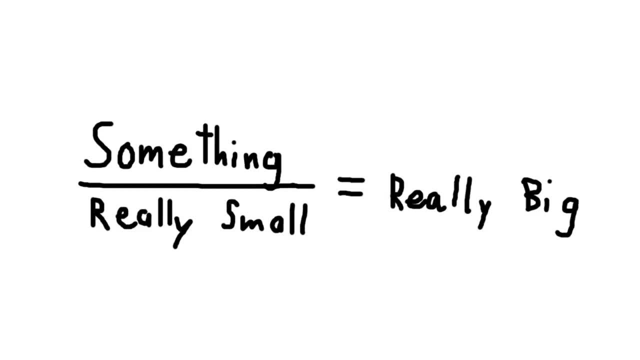 small number. Well, if we divide by a small number, we end up with a big number. So the result is officially a really big number. We can't really say infinity is the answer. but infinity is the answer. Now that we've learned about limits, let's go back to graphs. We want to know what the slope is at. 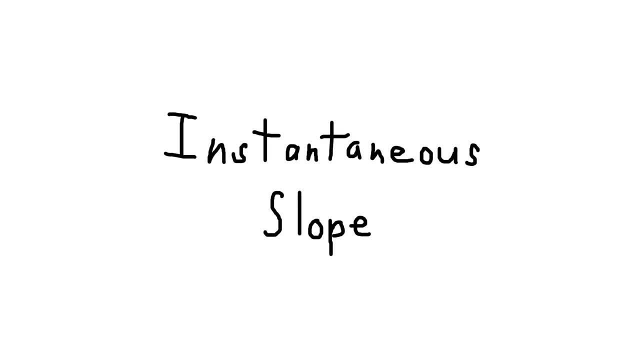 any given point on the graph. This is known as instantaneous slope because it changes to something else, the very next point on the graph. Let's look at a graph like: y equals x, squared At x equals zero. we can figure out the slope by looking at the points just to the left and right, To the left. 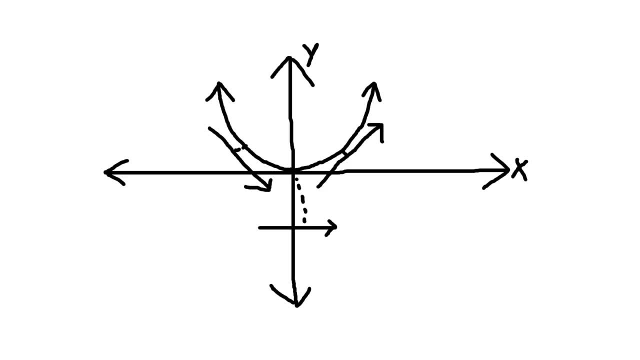 the curve goes down, so the slope is negative To the right. the curve goes up, so the slope is positive to the right. So we know that the slope in between the two must be zero, since the graph is continuous. Continuous just simply means that it's possible to draw the graph without ever picking up the pencil. 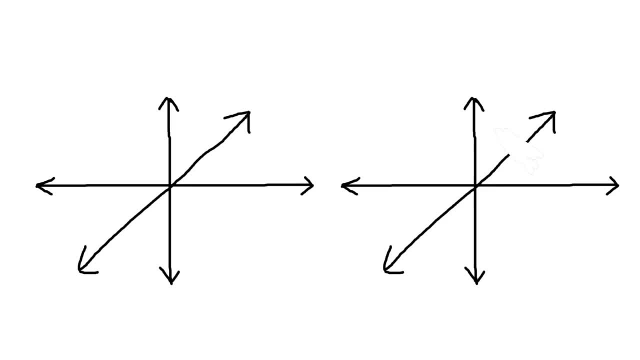 that you used to draw it. The graph on the left is continuous. The graph on the right is not. Any polynomial expression creates a continuous graph. y equals x, squared being one example. But what if we wanted to get the slope of any point on the graph To do? 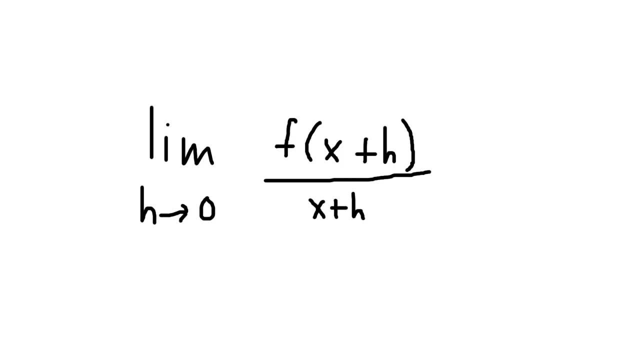 this, we take the limit as x approaches zero of the function evaluated at x squared and we get the slope of any point on the graph. To do this, we take the limit as x approaches zero and we get the slope at the x root of the equation. 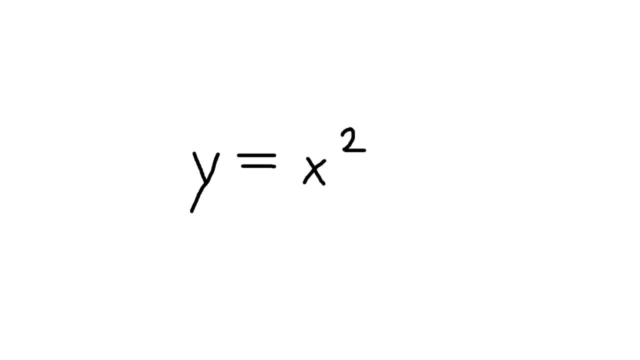 If the term is a constant, it becomes zero. If a term has a variable in it, we reduce its power by one and then multiply by their power as a constant factor. So x squared when derived becomes 2x, 2 is the. 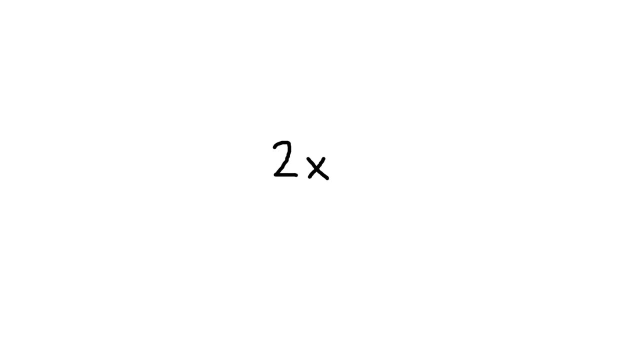 constant because 2 was the original power and the power becomes 1 because that's 1 less than 2.. Finally, after deriving a term, if the result is not 0, you must add an indicator that you have derived it, For example y when derived. 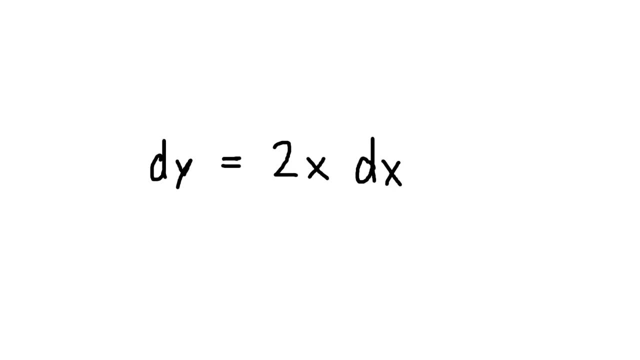 becomes dy read as the derivative of y, x squared, when derived becomes 2x, dx- 2x from the rules we mentioned before and dx as an indicator that this term has been derived. Another important note: d is not a variable, it is just a letter. 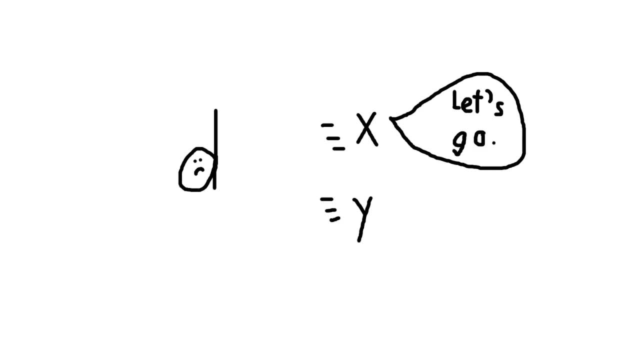 put in front of another variable to indicate that it's been derived. So our final equation is dy equals 2x dx. We can clean this up one more time by dividing both sides of the equation by dx. This gives us dy. dx equals 2x This. 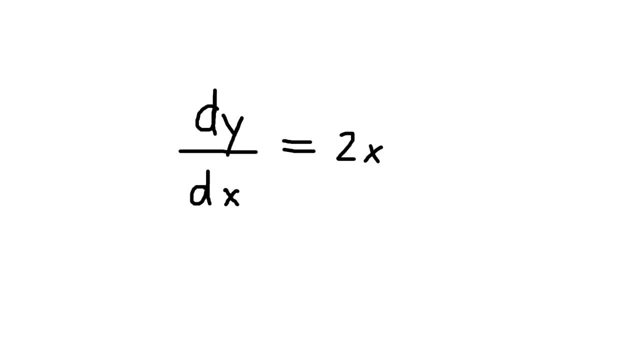 is read as the derivative of y in terms of x is 2x. So now, what do we do with 2x? Well, we can now plug in any value for x and we can find out the slope of the graph. y equals x squared, So if x equals 7,, then dy equals 2x. So now, what do we do with 2x? Well, we can now plug in any value for x and we can find out the slope of the graph. y equals x squared. So if x equals 7, then 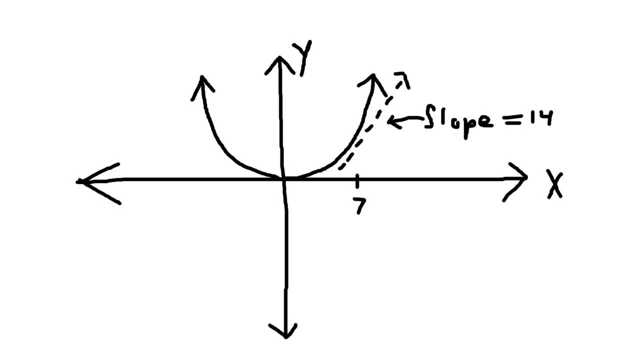 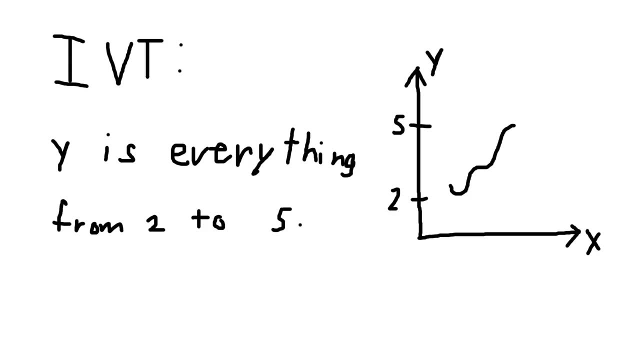 then 2x equals 14.. So the slope of the graph at x equals 7 is 14.. The intermediate value theorem pretty much says that if I draw any continuous curve, point out where the biggest and smallest y values are, the graph must contain all the y values in between. If that wasn't true, 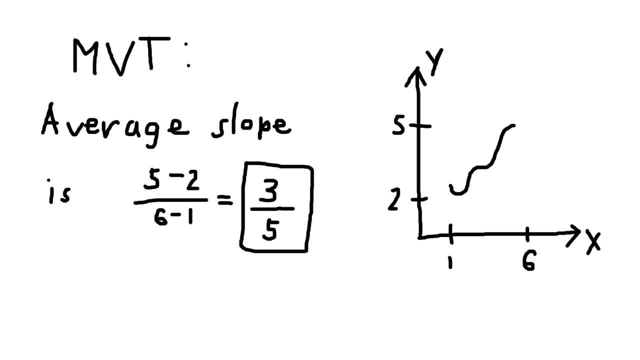 Limbo would be a really easy game: Just walk through the missing part of the stick. The mean value theorem states that if I have a continuous curve and a section of the curve is differentiable, then at that section of the curve the weighted average slope is the slope.